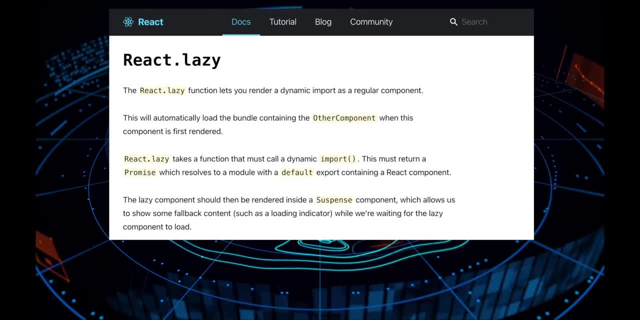 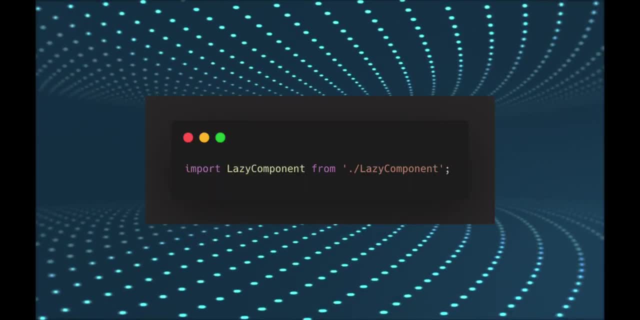 only when the application is running. You may also use React Suspense and React Lazy for lazy loading when it's needed. React comes bundled with the React Lazy API so that you can render a dynamic import as a regular component. So instead of loading your regular component like this: 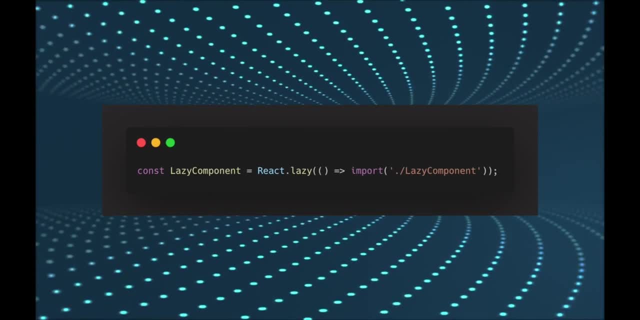 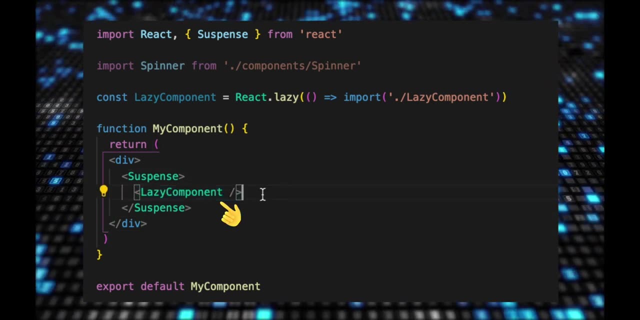 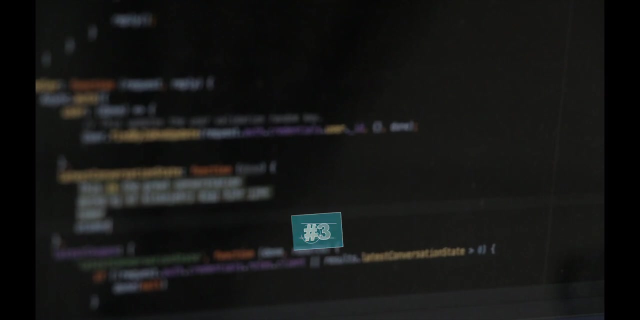 you can do it like this: to cut down the risk of performance: by using the lazy method to render a component. Lazy component is typically rendered inside a Suspense component, which allows you to add a fallback content as a loading state while waiting for the lazy component to load. Tip 3,. 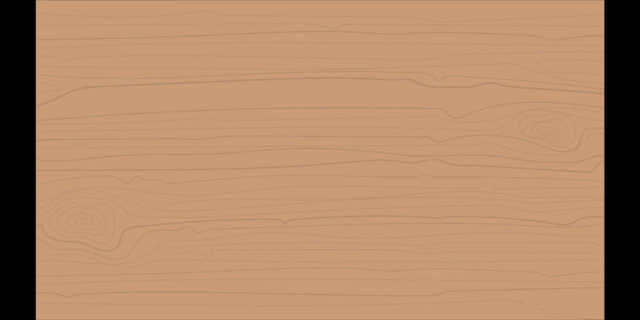 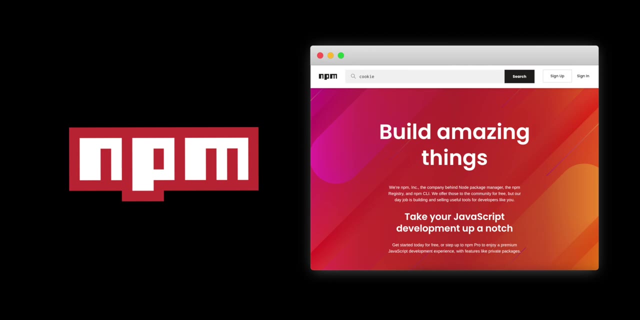 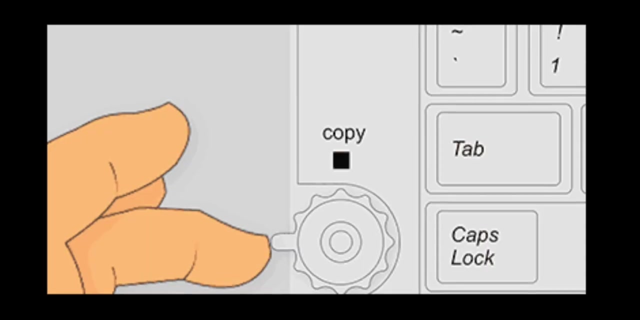 dependency optimization. One of an overlooked aspect of software development is how much programmers rely on open source libraries and packages for ready-to-use code. Sometimes it is a little too much, Instead of writing code from scratch, or even copying and pasting code from one. 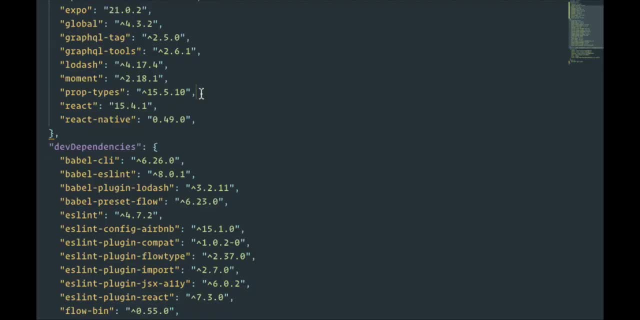 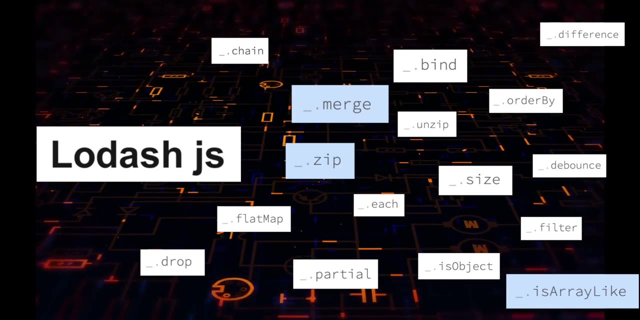 program to another. some programmers still rely on what is called a dependency, For example the Lodash library. Let's say we only need 3 of the 100 methods from this library and create a new one methods from the library. Having all extra methods in the final bundle is not optimal. 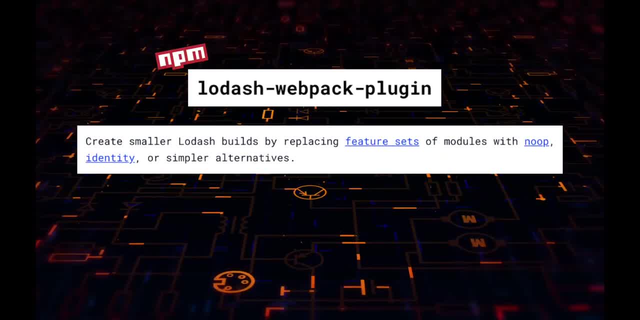 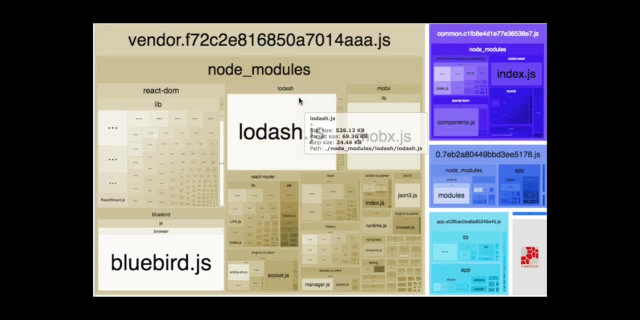 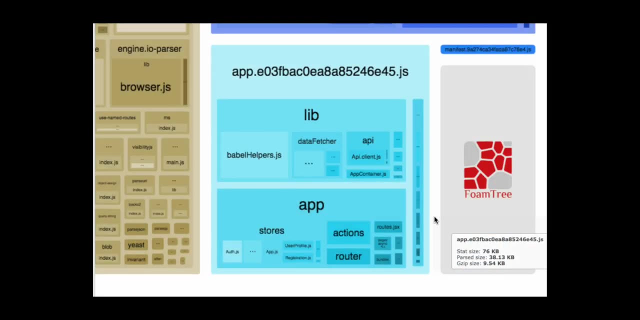 We may use Lodash Webpack plugin to remove unused function and customize a build. for us, This will produce a smaller build of the library. It's worth checking how much code you are actually utilizing from dependencies when optimizing the application bundle size. Also, it is a good idea. 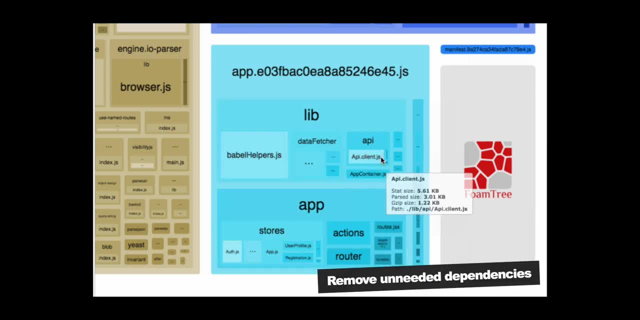 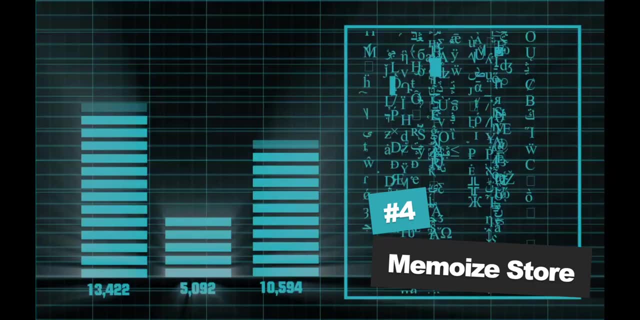 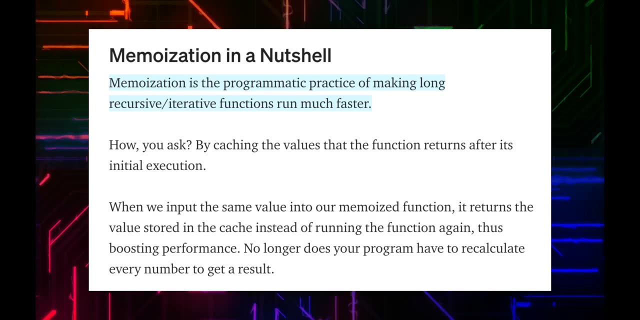 to monitor and remove dependencies that is no longer used. Sometimes the best dependencies is no dependencies at all. Tip number four: Memoize. store Frequent interacting with a store. retrieving the same data is redundant and needs to be avoided. Memoization is a technique that 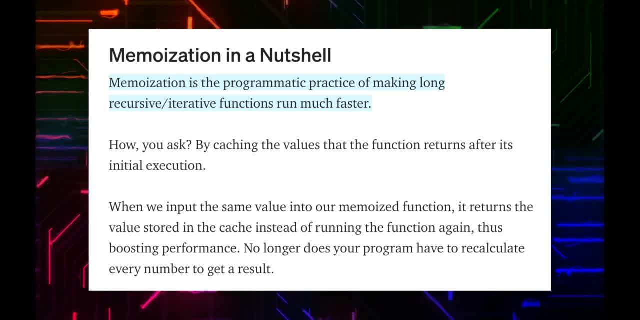 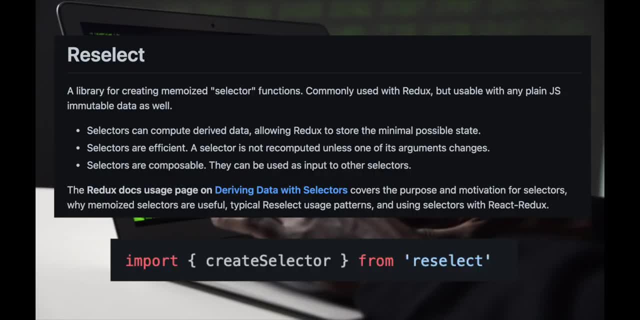 is often applied to the application, but it can also be applied to store like Redux and other state management libraries. For example, reselect library exports, create selector- that would generate a new library. This is a good idea to monitor and remove dependencies. that is no longer. 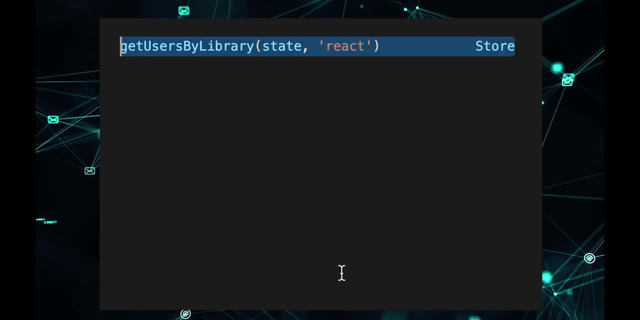 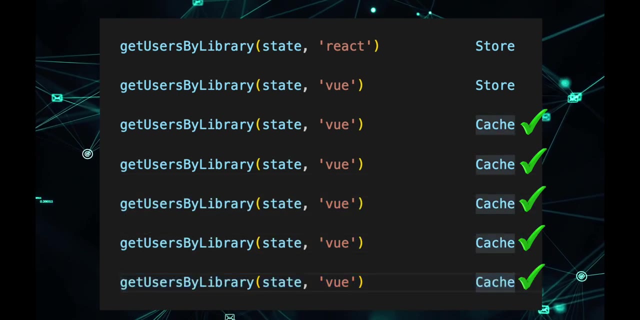 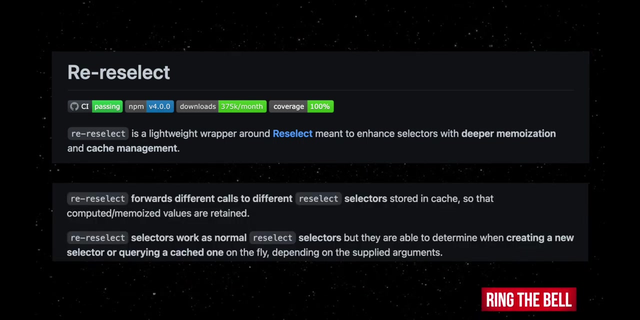 These selectors will remember the arguments passed in the last time it was invoked and it doesn't recalculate if arguments are the same. Re-reselect would take this further. if deeper memoization and cache management is required, This will solve the issue with reselect as it. 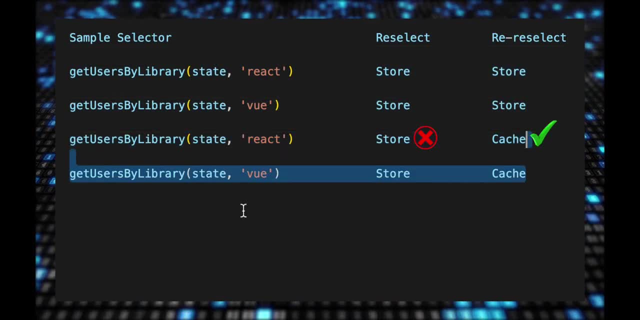 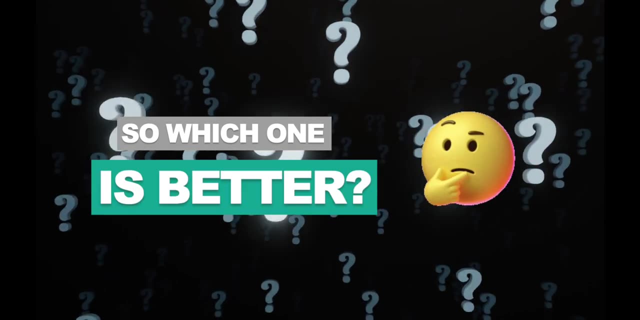 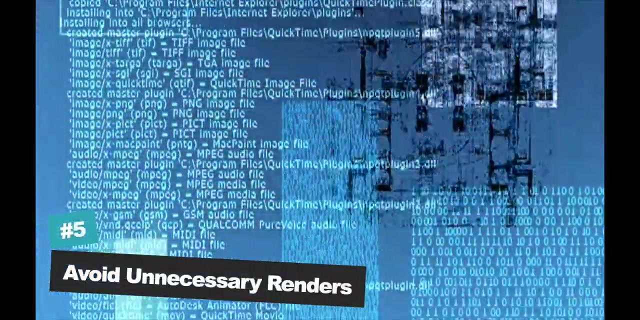 has a caching limit of one, which means switching between different arguments using standard reselect selectors causes cache invalidation. Both of these libraries offer great solution for caching, but you may choose the solution that depends on your use case. Tip number five: Avoid unnecessary component. renders Unnecessary re-rendering. React component is a common problem. 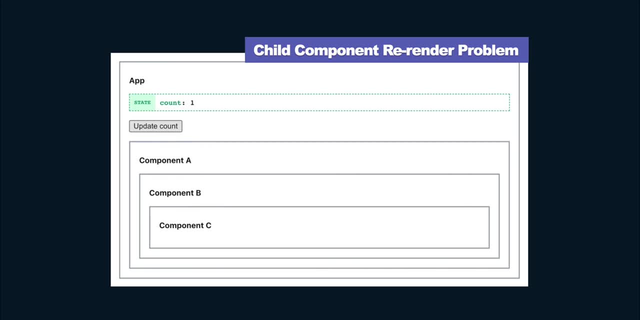 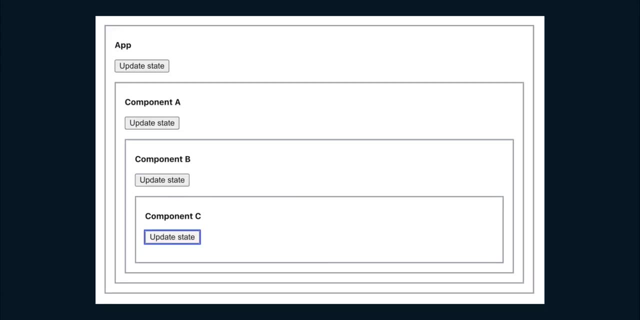 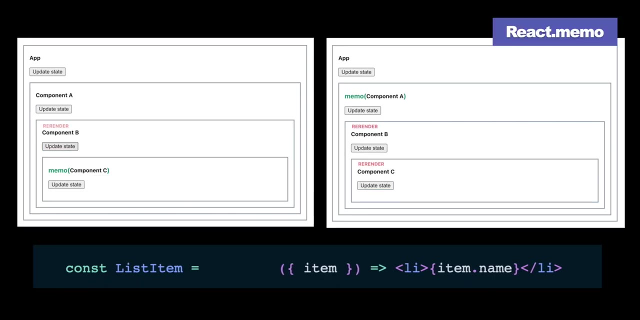 in React. When a component re-renders, React will also re-render its child component by default. This will slow the app and make the user of the app frustrated. No one wants to use an app that is laggy and feel unresponsive. To prevent this from happening, functional components can use: 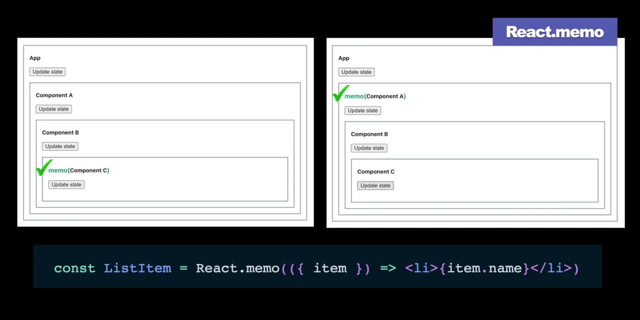 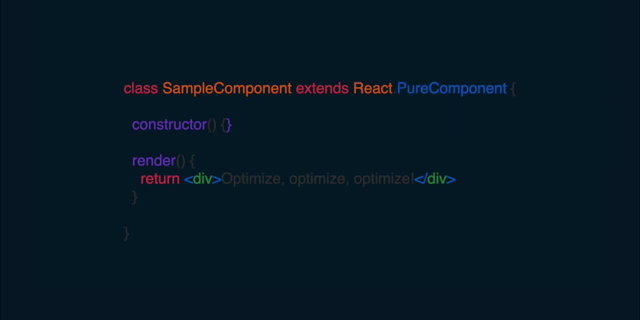 React memo to ensure the component is only re-rendered when its props change. Class-based components can utilize React pure component to get the same effect. Also, you can return false from should component update instead if you know that in some situation that the component doesn't. 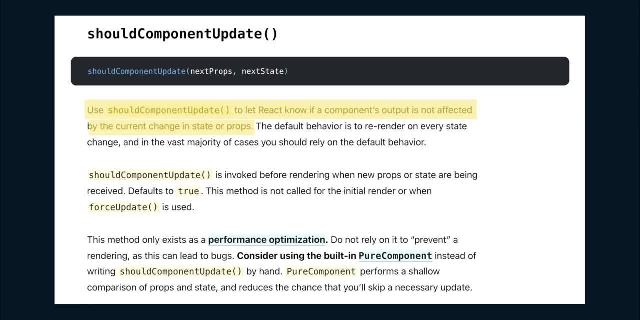 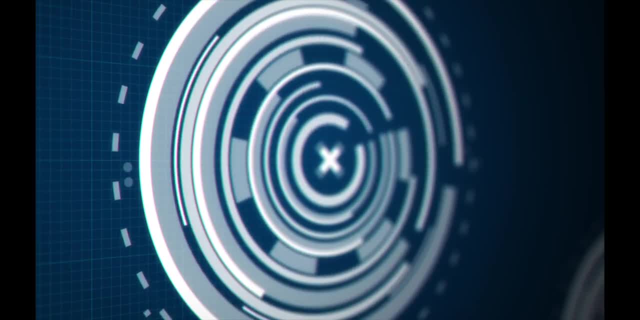 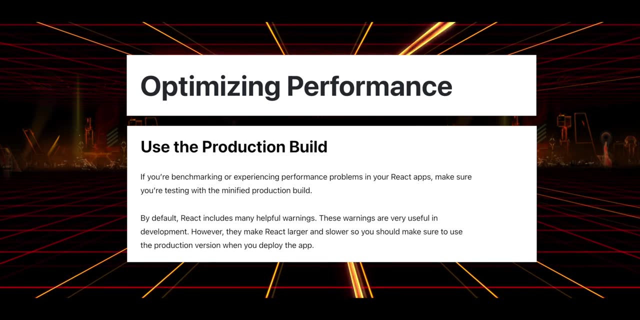 need to update to skip the whole rendering process, including calling render on components. Tip number six: Use production. build React includes many helpful warnings that are very useful in development. by default, However, they make React larger and slower, so you should make sure to use. 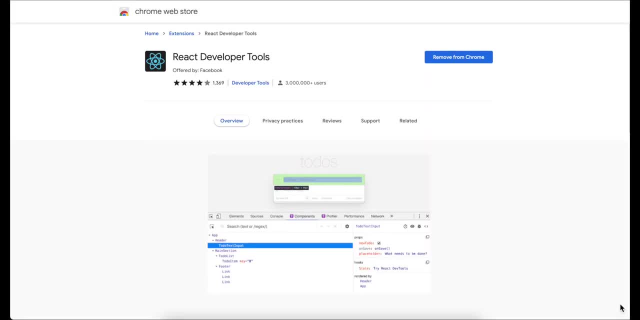 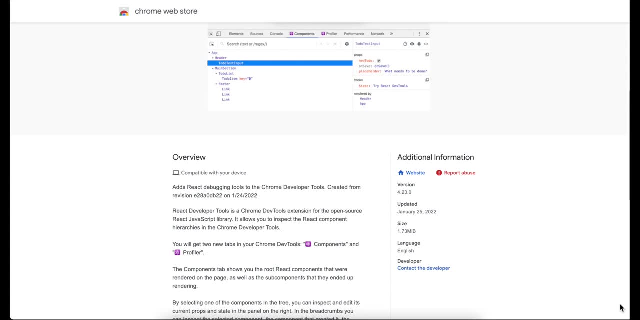 the production version when you deploy the app. Installing React developer tools for Chrome is a good extension to verify if your build process is set up correctly. If you visit a site with React in production mode, the icon will have a dark background. React in development mode will. 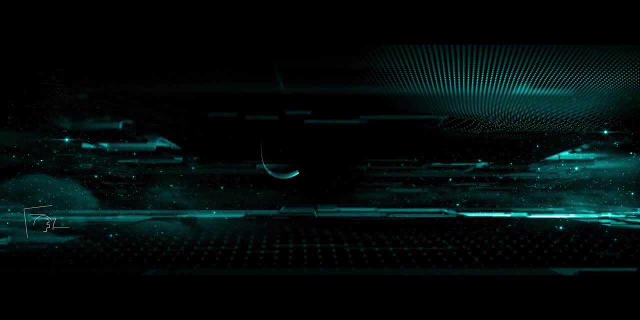 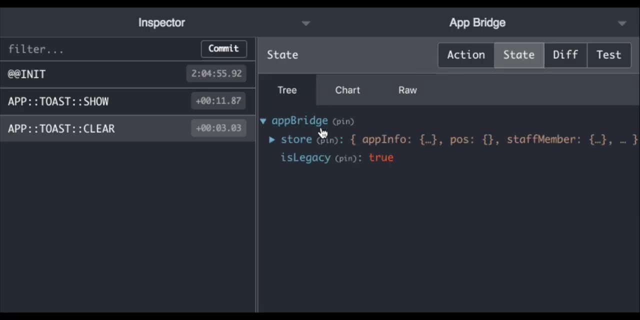 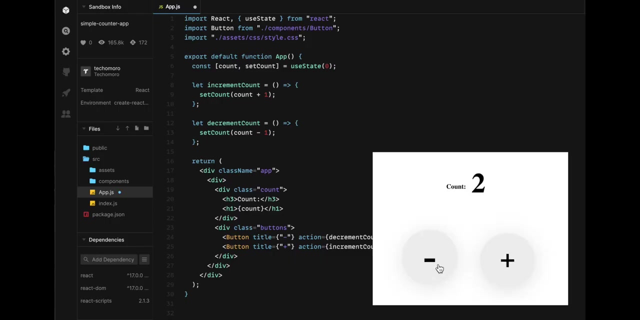 have a red background on the icon. Tip number seven. Keep state local instead of store. It is easy to get carried away and dumping most of the state of the application to state management libraries. Keeping the state to the component locally is preferable and will always be faster. 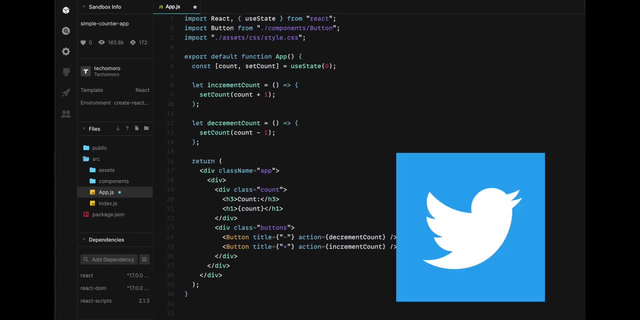 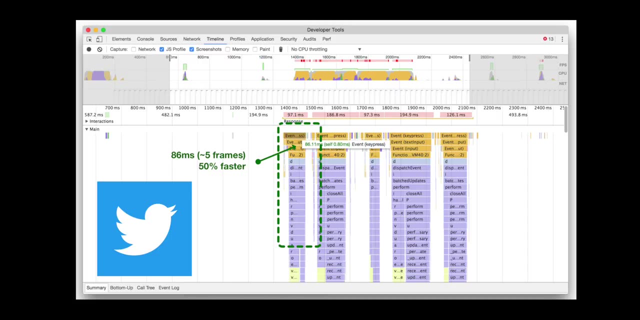 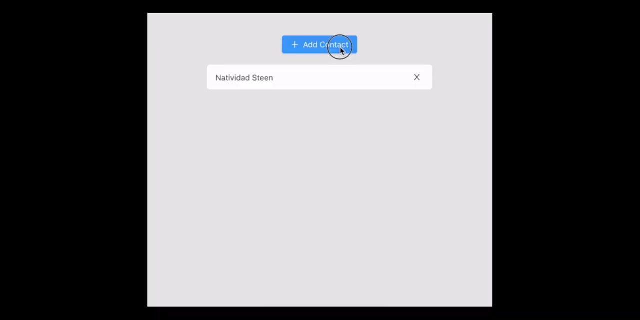 than using a global store. Twitter knows this very well. This one optimization alone reduced their overhead by 50%, which is drastic and good for users of their app. While this may not hurt desktop computer much, a small mobile device will take an obvious performance. hit Before storing a. 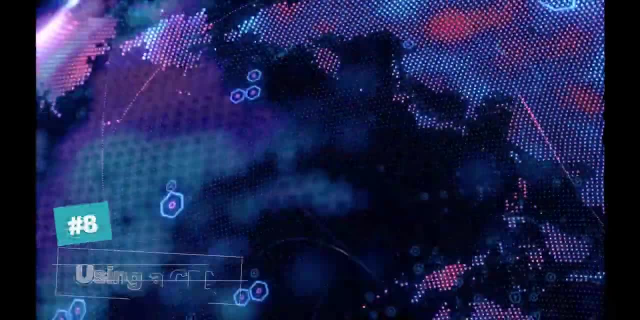 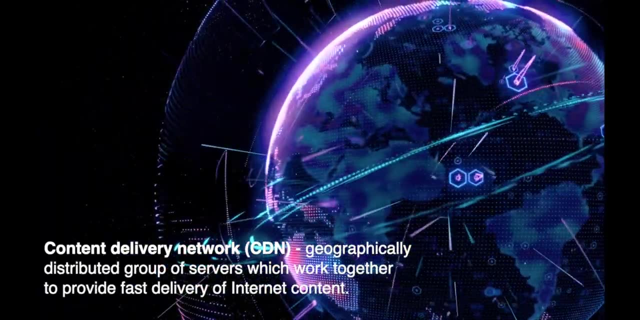 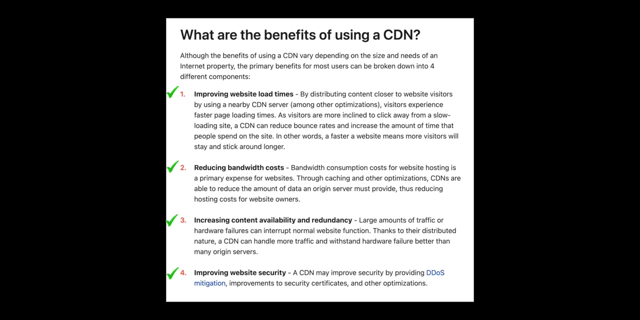 file, always check if it can be avoided. Tip number eight: Using a CDN. A CDN is a great way to deliver static content to your audience more quickly and efficiently. Having content delivered by CDN will reduce bandwidth costs, improve page load times and increase global availability of. 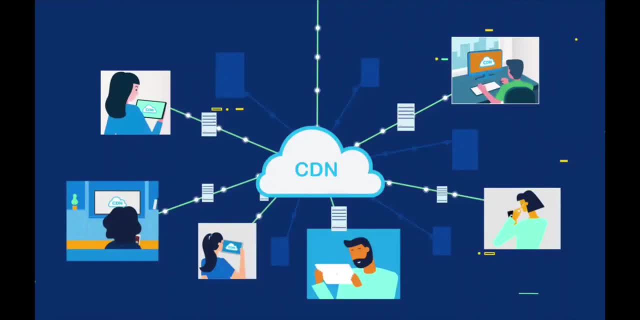 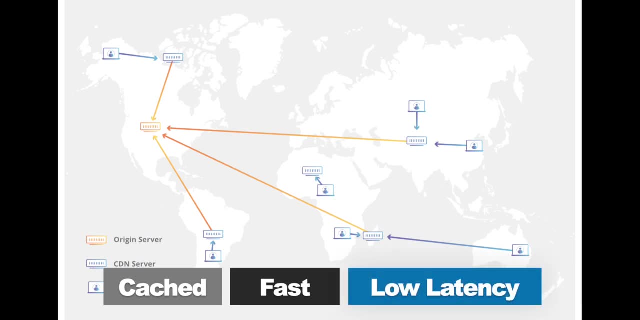 content. ReactJS applications will tremendously benefit from CDN, as they will receive files from a server that is geographically close to them, cached fast and have very low latency. The best and fastest ReactJS application will look slow if the servers cannot speed. 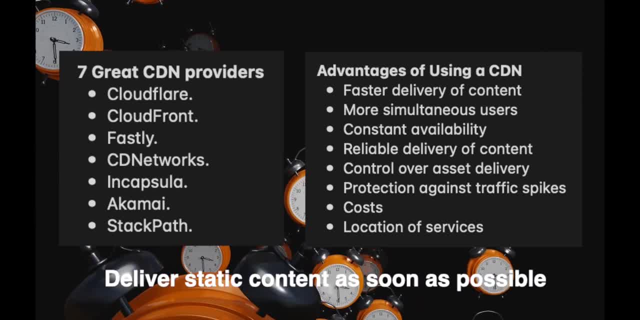 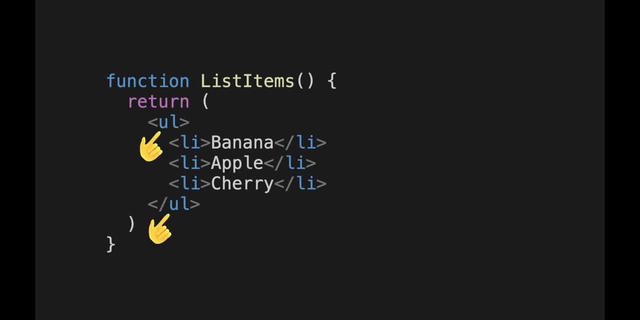 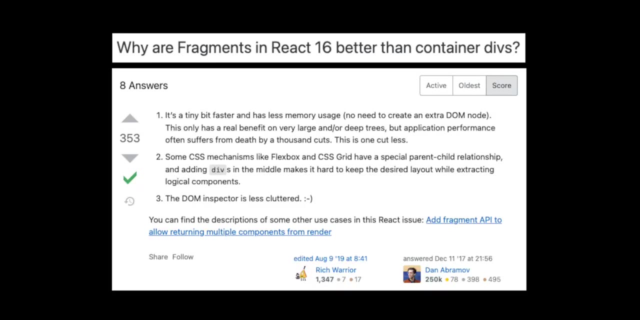 up the delivery of static content to the users. Tip number nine: React fragments. React requires a surrounding container for every component we create. From version 16.2, it is no longer needed because of React fragments. Fragments avoid creating an extra unnecessary. 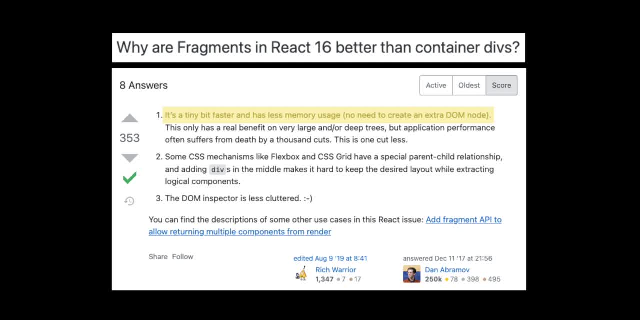 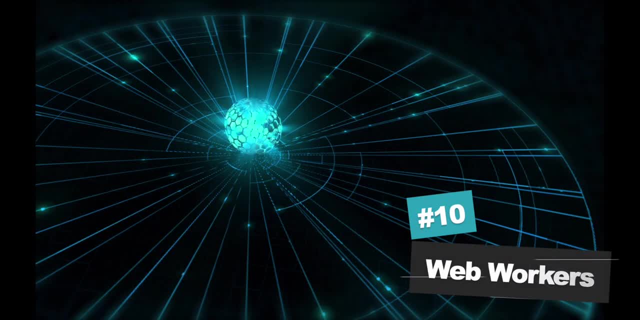 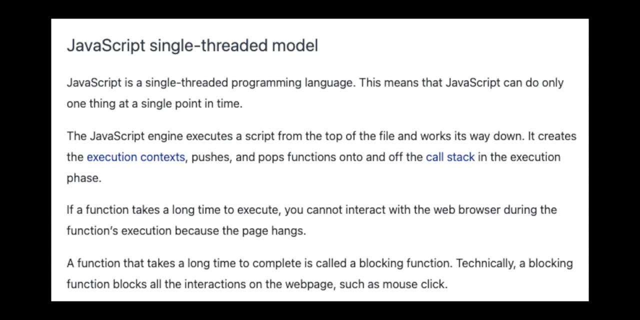 DOM node, which is good for memory. Every little nodes that we can save adds up easily, making our React application cleaner and speedy. Tip number 10. Using web workers. Extensive tasks or operations can block the execution of an app. JavaScript is a single. 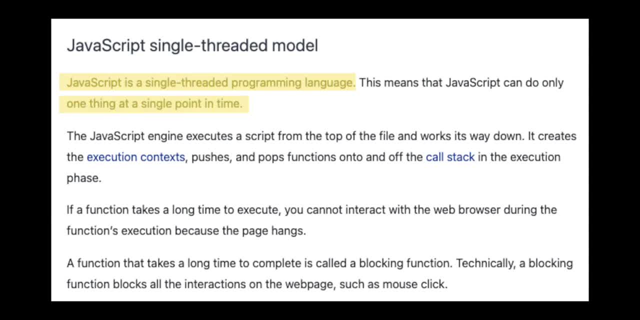 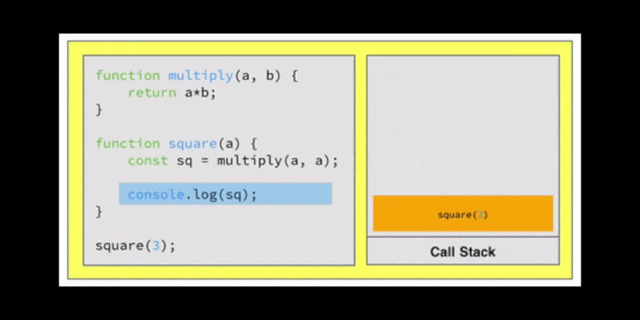 threaded language which executes one statement at a time. That means script or code must finish executing before moving into the next. React is not an exception to this rule. Web workers make it possible to run a process in web applications background thread, separate from the single. 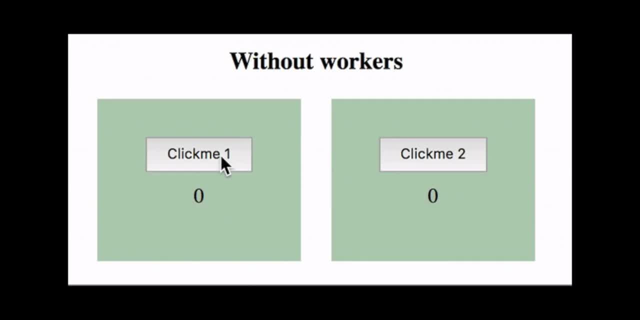 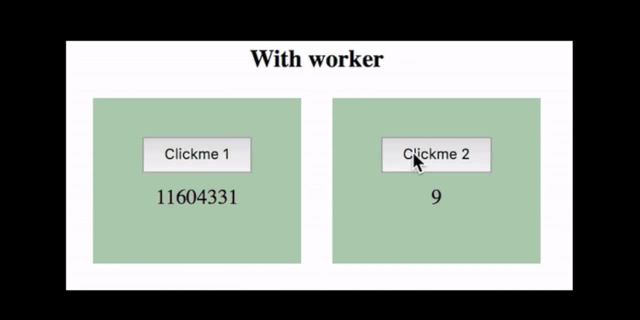 execution thread, Our program is able to run without being blocked or slowed down to achieve parallel compute by performing the laborious processing in a separate thread. React applications can take advantage of web workers to delegate extensive tasks in the background, as it will not affect page performance. 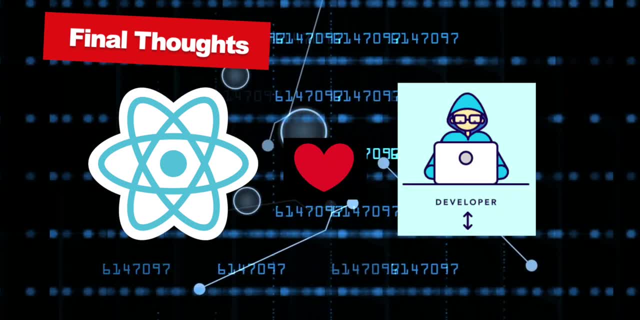 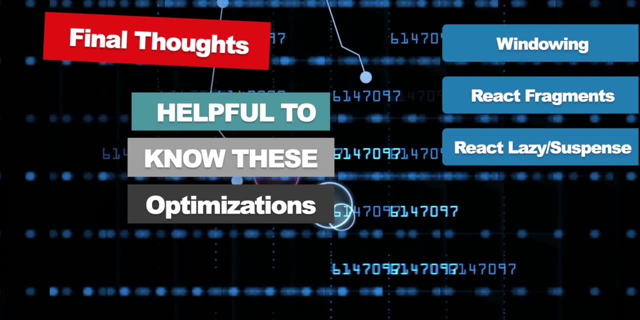 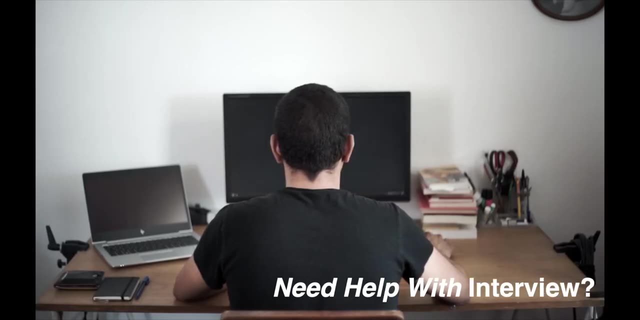 React uses several clever techniques to ensure the app we create is performant. Not everything is free, so we also have to be mindful of things that may slow ReactJS, like excessive re-rendering and other areas. If you are in the job market and need some refresher with React, I created a couple of 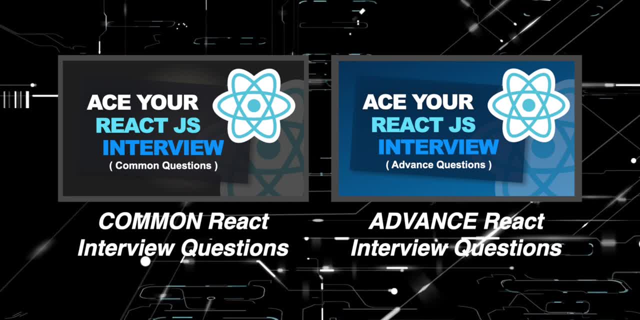 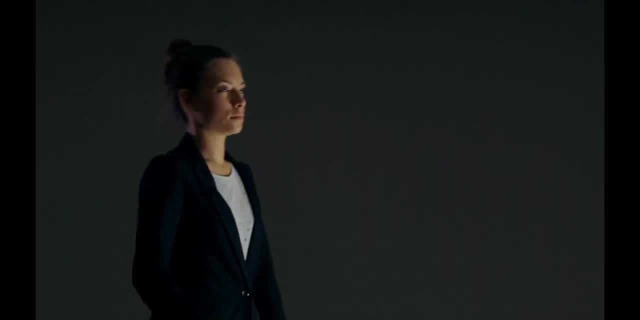 videos for the most commonly asked questions being asked in an interview. Also, here is a video to help you get ready for the coding part of the interview. I hope that you find these optimizing techniques useful. If you are new to this channel, please like this video and subscribe to my channel.